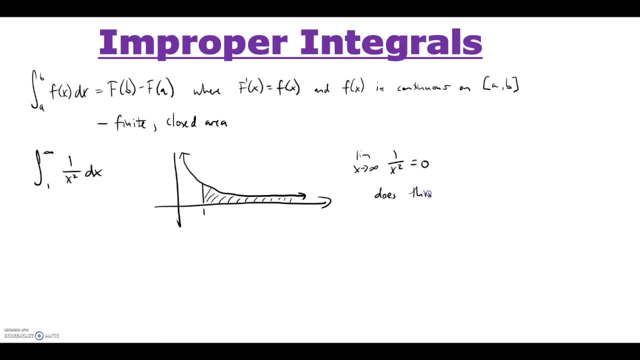 that means in terms of the area under that curve. So the question becomes: if the limit of this function as x approaches infinity equals zero, does that mean this area eventually closes? Or to think about this question in another way, if the limit as x approaches infinity equals zero, does this mean at large enough values of x at some point does area stop being added to this region? And this brings us to the concept of an improper integral. 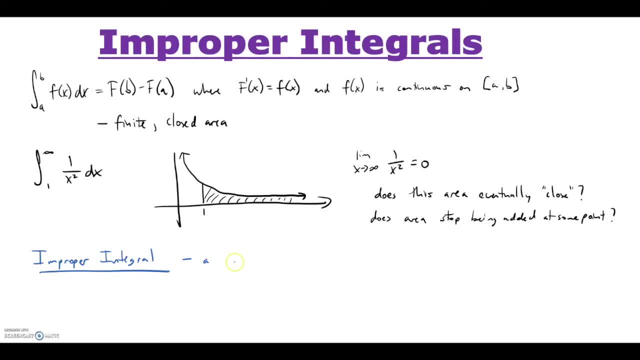 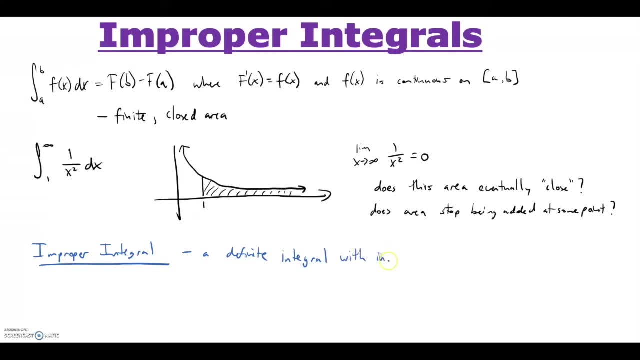 And an improper integral is a definite integral, with infinity serving as at least one boundary on the integral. But there's one major issue with improper integrals, and that is infinity is not an actual number. So to calculate an improper integral, we calculate those using limits. Since infinity is an improper integral, we calculate those using limits. 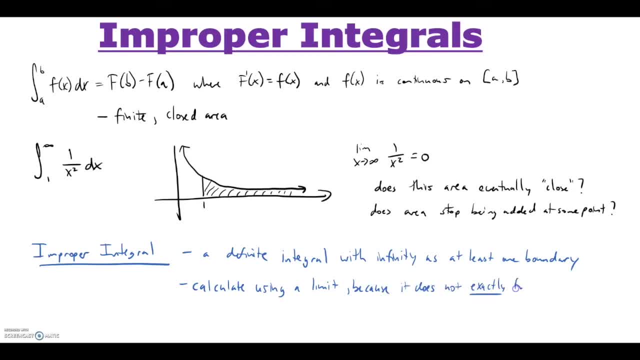 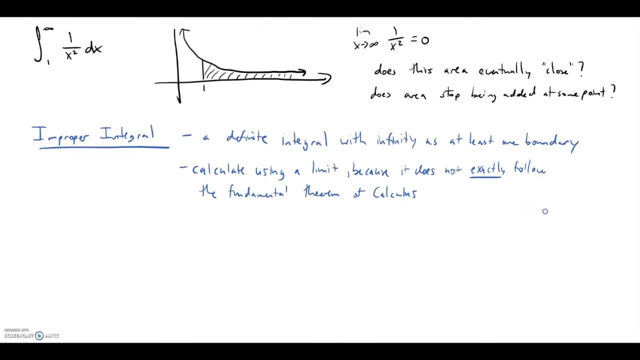 so when this is not an, it is not a defined value, then these integrals do not exactly follow the fundamental theorem, Calculus, which requires both boundaries to be constant numbers. And so now let's see how this process will work. Let's go back to that simple example: the integral. 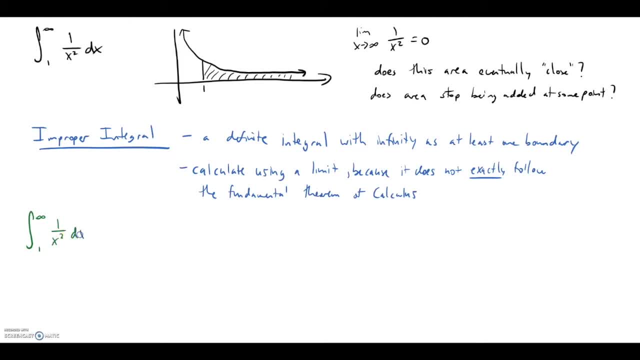 from one to infinity, of one over x squared with respect to x. And what we're going to do is we're going to set this up as the integral from 1 to b of 1 over x squared, dx, where b is a constant value, and let b approach infinity using 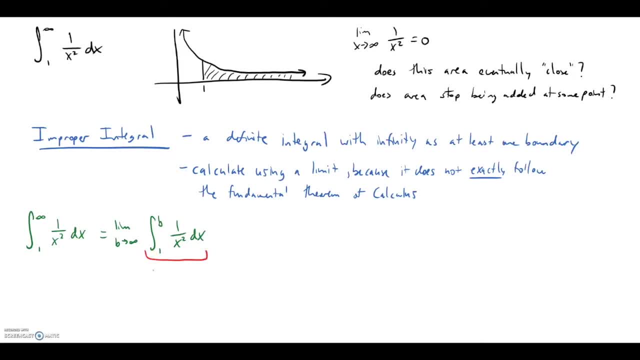 a limit. And now, looking at our definite integral, we've solved one issue. Both boundaries 1 and b are constants. We already know that 1 over x squared is continuous from 1 to any larger value b. So this definite integral will follow the fundamental theorem of calculus, which means: 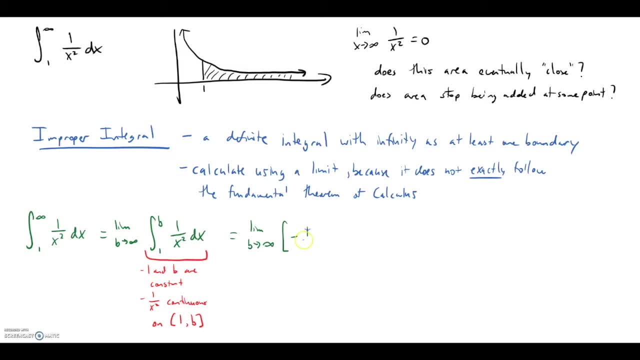 we can evaluate it. This will be the limit as b approaches infinity of our antiderivative negative 1 over x, evaluated from 1 to b, which will be equivalent to the limit as b approaches infinity which is negative 1 over b, minus negative 1 over 1.. 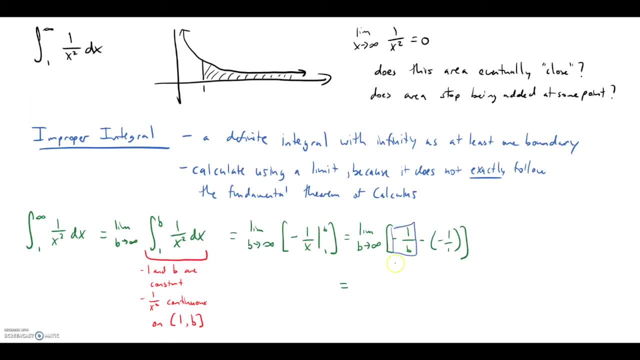 And notice this negative 1 over b. if we let b approach infinity, that term will approach zero And the negative of negative 1 over 1 will be a plus 1.. So this limit and subsequently the integral from 1 to infinity of 1 over x, squared with 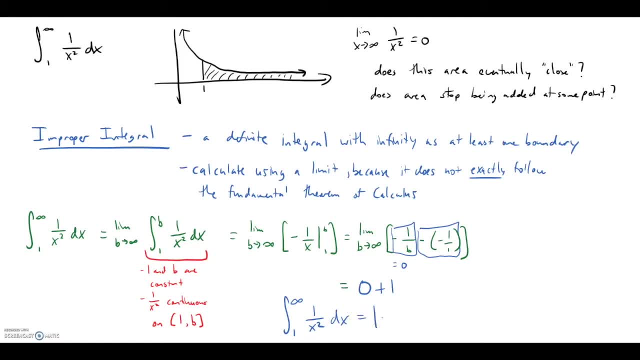 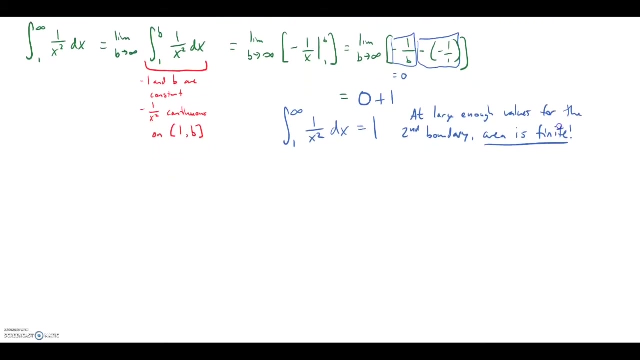 x will equal 1.. Which is a somewhat surprising result. At large enough values for x or at large enough values for the second boundary on our definite integral, the area actually becomes finite, Or the other term that's going to start coming up is the area converges to one single value. 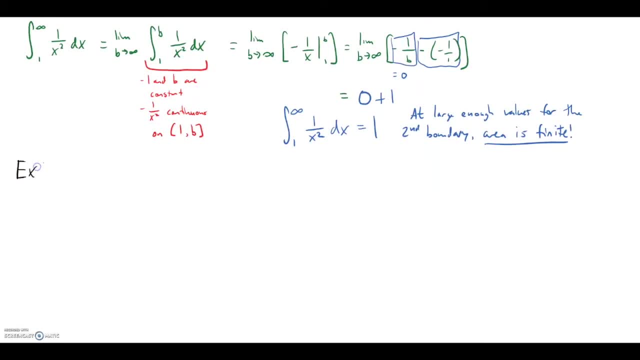 So let's finish by taking a look at one more example as a contrast to that first situation. So let's finish by taking a look at one more example as a contrast to that first situation. So let's finish by taking a look at one more example as a contrast to that first situation. 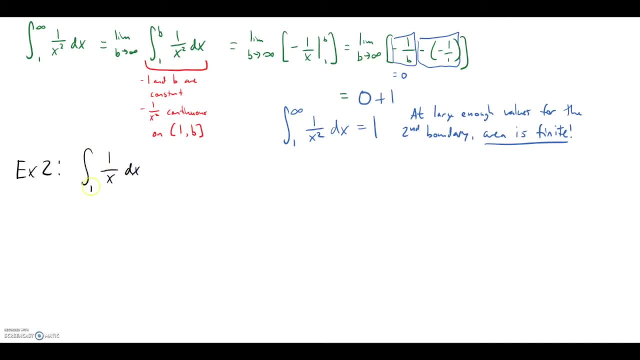 And in this example we'll look at the integral for 1 over x, dx also from 1 to infinity, like we saw in the first example, And we'll solve this by setting up the limit as b approaches infinity for the integral from 1 to b, of 1 over x with respect to x. 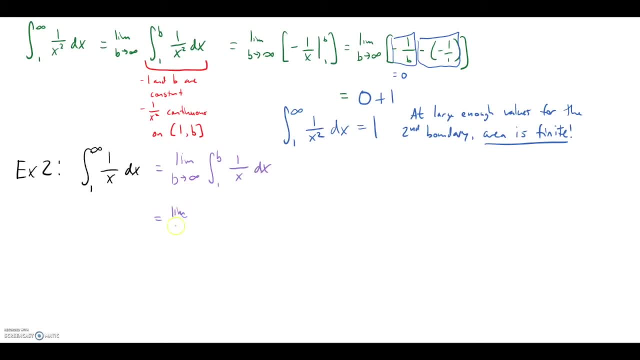 The function now has constant boundaries and 1 over x is continuous from 1 to larger values of x. So we can evaluate this for our antiderivative, which in this case is ln. So this will be the limit as b approaches infinity for ln.